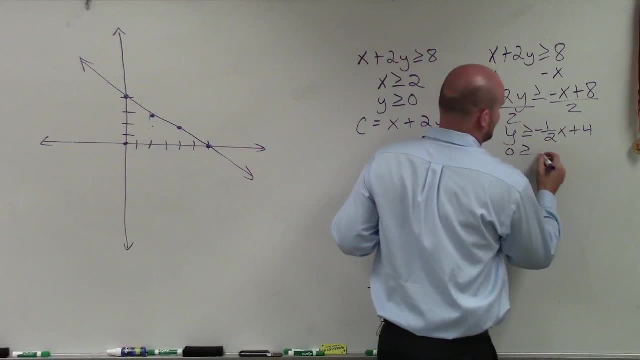 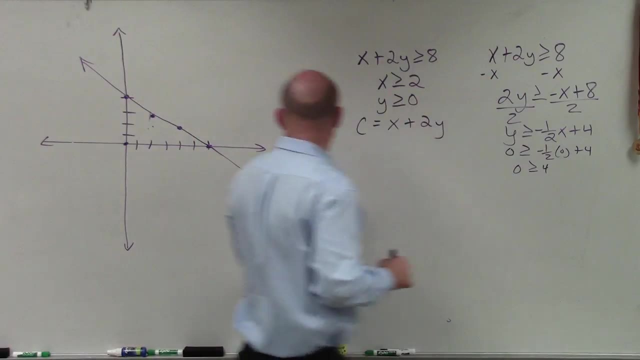 use 0, 0, and I'll just plug in my test point to determine if I'm shading up or down, And I can see 0 is greater than or equal to 4, which of that is false. so therefore, my feasible region is going to be facing up above this boundary line. 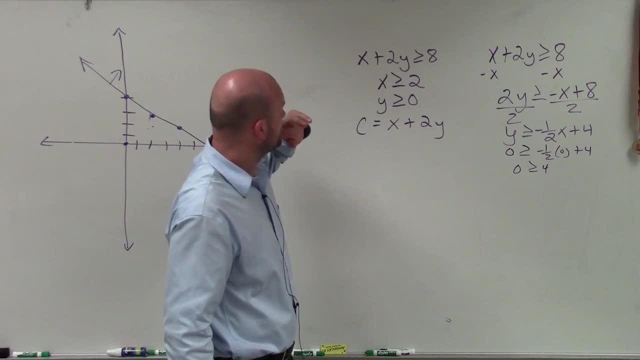 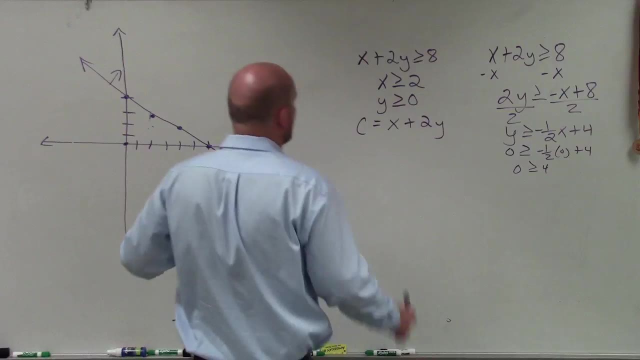 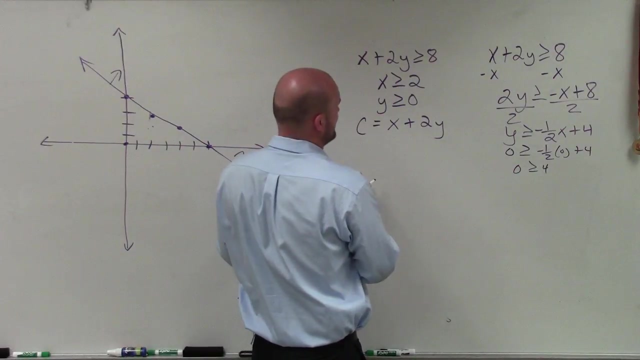 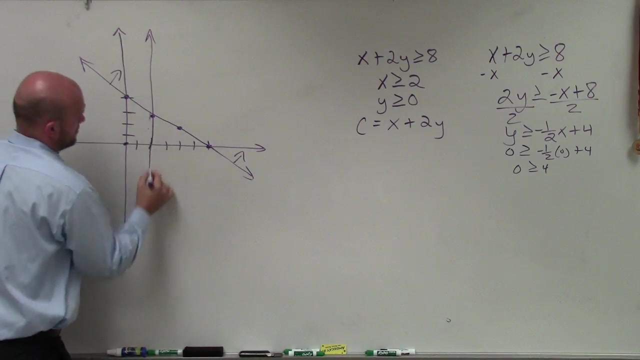 My next two: Y is greater than, Y is greater than or equal to, okay, So I have that all set and that is false, so we're going up. Then my next two is: y is greater than 2.. So to graph that: or x is greater than 2, so I'm going to go over to 2, graph this line. 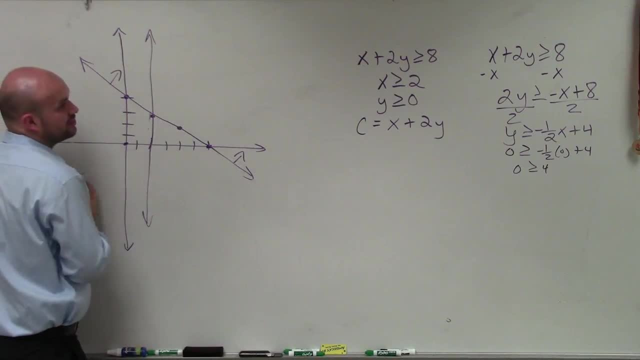 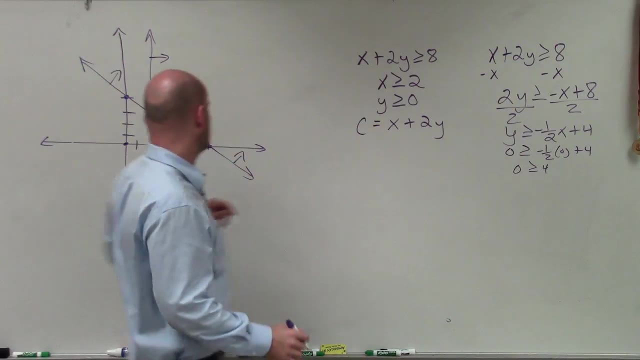 And since x is greater than that's going to be all the values that are going to be going to the right. So that's going to be x. Okay, That's going to be feasible regions that are going over to the right. And the last one: y is greater than 0.. 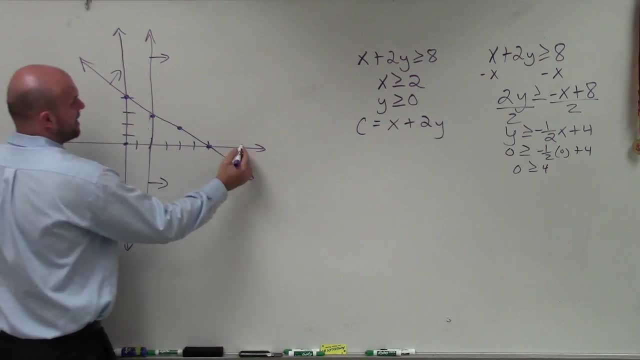 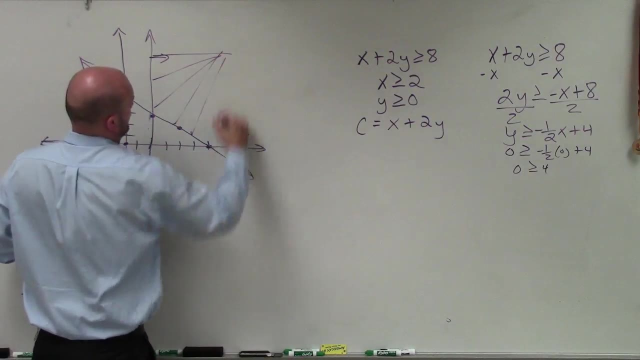 And that is going to be my y-axis, and values that are greater than my y-axis are going to be going up. So therefore, you can see that my feasible region here is going to be all this area, Continually going up, continually going over. 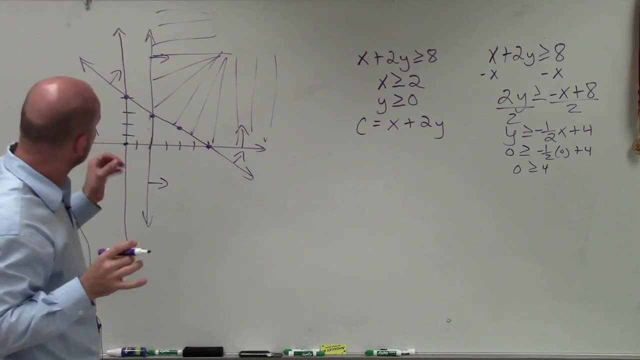 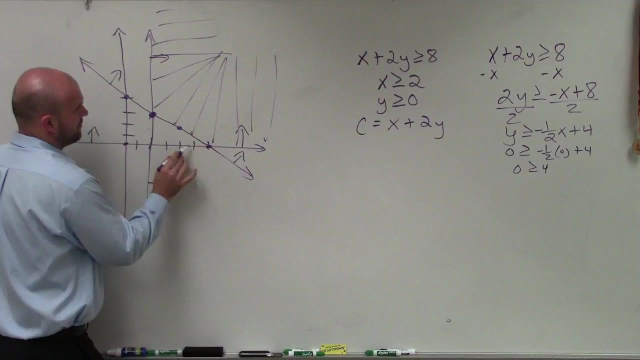 And there's three. actually only two vertices that I have here is right here and right here, And those two vertices are 1, 2,, 3,, 4,, 5, 6, 6, comma 0, as well as 1, 2,, 1, 2, 3, as well. 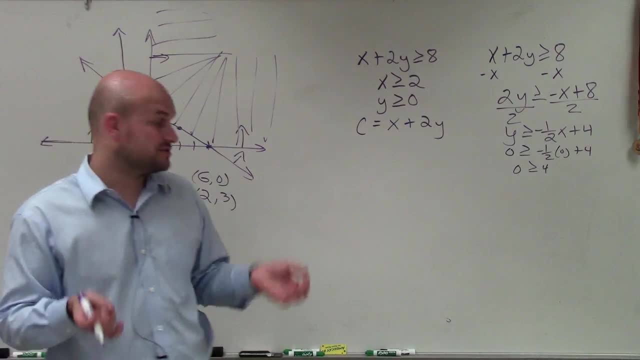 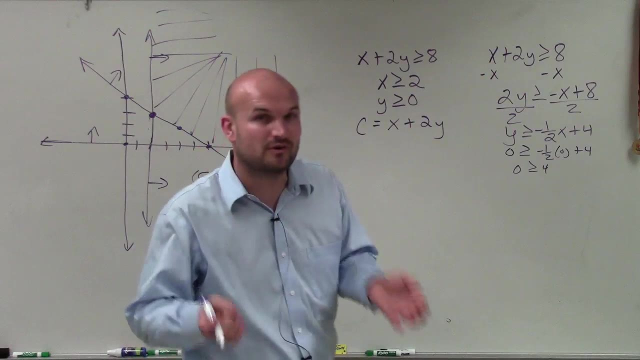 as 2 comma 3.. So now to go ahead and test these in my objective functions, I'm going to take these two vertices and I'm going to plug them into my objective function to be able to determine what is going to provide the minimum cost for my feasible region. 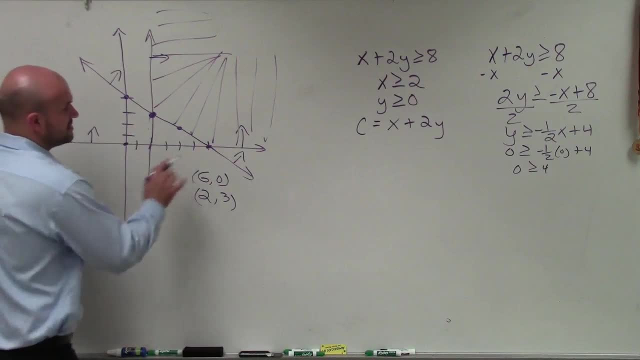 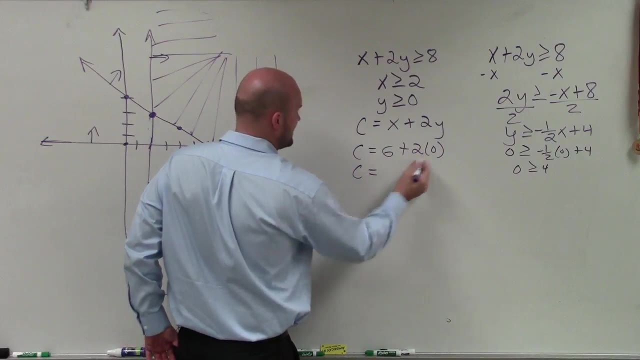 So therefore, I have 6 comma 0. I'm going to plug this in, I'm going to plug this in. I'm going to plug this in. So I'll say: c equals 6 plus 2 times 0. And that is c equals 6.. 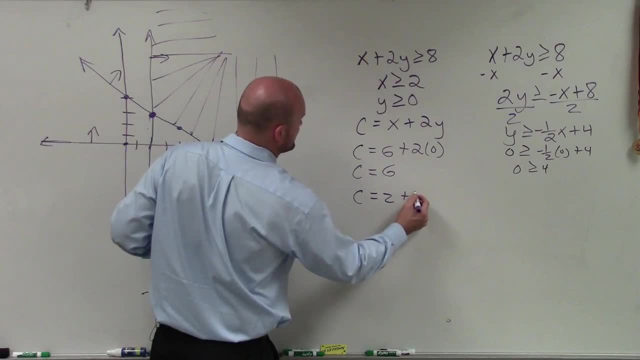 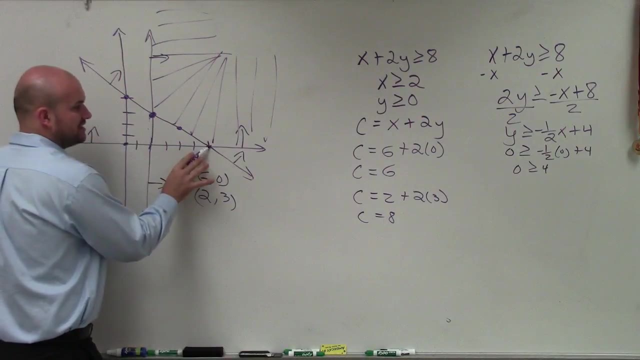 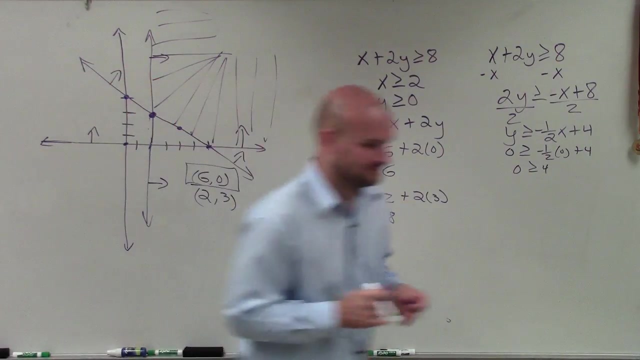 And then my other one I'll plug in: c is equal to 2 plus 2 times 3, where c equals 8.. So, therefore, this value is going to be larger than this value, And again I'm looking for my minimal point, which will be 6 comma 0.. 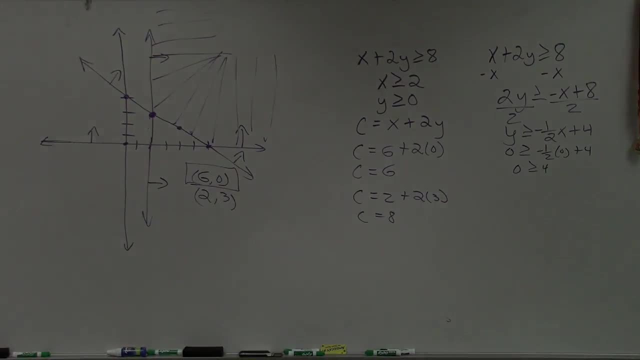 Thanks, Thank you. CLOSED CAPTIONING PROVIDED BY WKNO-MEMPHIS. The video sanitizer was disconnected during production. May this and that be. 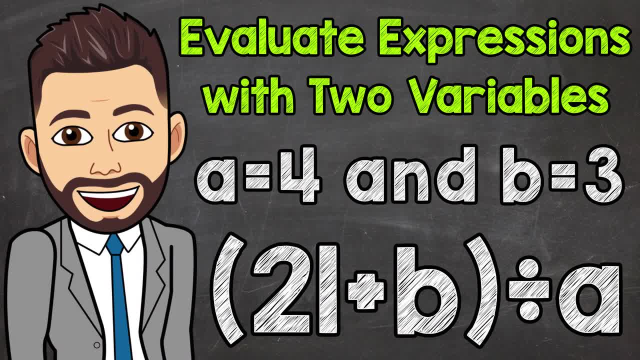 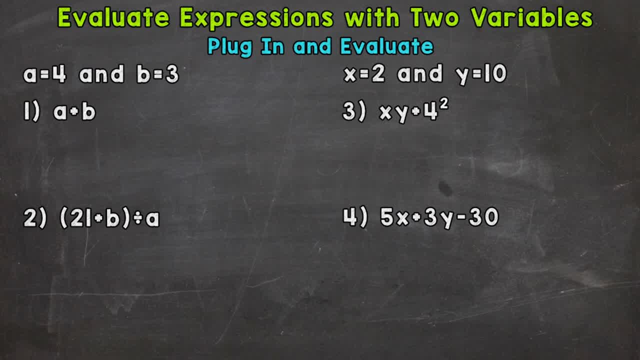 Welcome to Math with Mr J. In this video I'm going to cover how to evaluate expressions with two variables and we have four examples that we're going to go through together in order to get this down. So for numbers 1 and 2, we have a and b. a equals 4 and b is going to equal 3.. 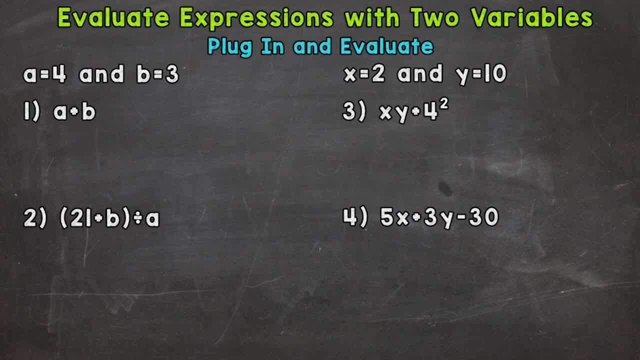 For numbers 3 and 4, we have x and y. x is going to equal 2 and y equals 10.. So let's jump into number 1, where we have a plus b. So we want to plug in the values for. 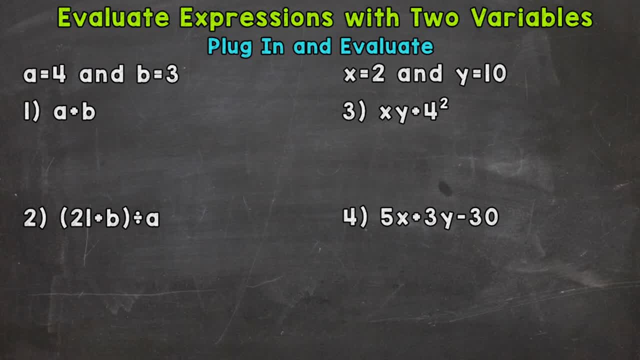 those variables- a equals 4 and b equals 3- and then evaluate. So let's rewrite our problem with the plugged in variables. So for a we need to plug in 4, plus for b we need to plug in 3.. 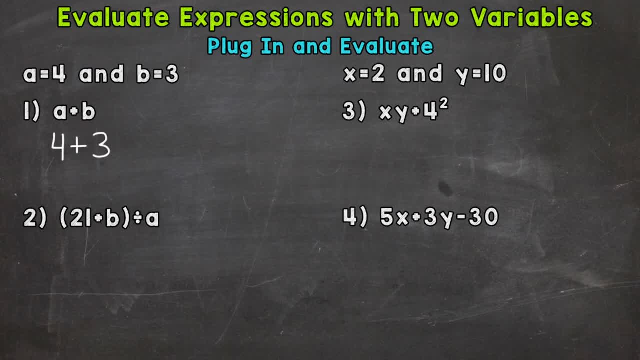 3. Now we evaluate. So 4 plus 3 gives us an answer of 7.. Let's go on to number 2, where we have parentheses 21 plus b, end parentheses divided by a. So let's plug in and evaluate: So 21 plus 3, end parentheses there. 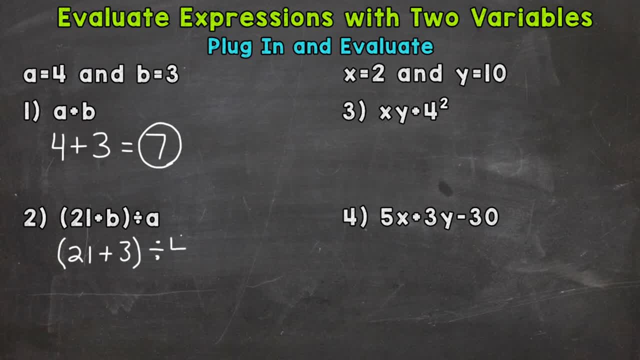 divided by a. So let's plug in and evaluate: So 21 plus 3 end parentheses there. divided by a, So 24 plus 3 end parentheses is divided by plug in 4 for a. Now, in this problem we have multiple operations and steps, So we need to use the order of. 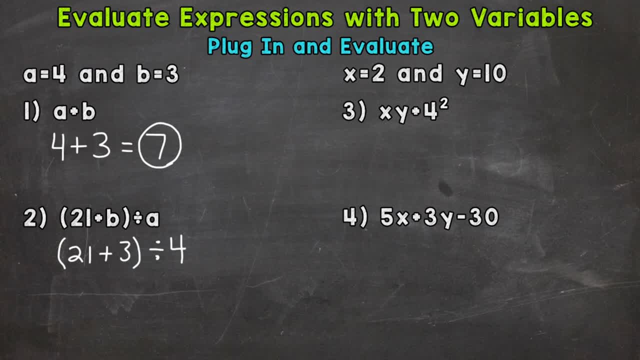 operations. So any parentheses? Yes, that's where we need to start. We have 21 plus 3 in the parentheses, So that's going to give us 24.. Bring down everything we did not use, So the division sign and the 4..